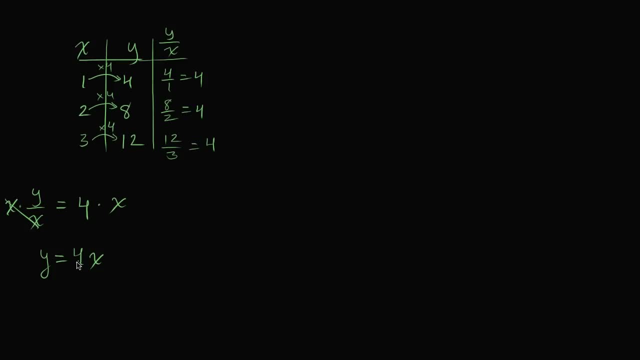 We are multiplying by four, And so four in this case, four in this case, in this situation, this is our constant of proportionality, Constant, constant. Sometimes people will say proportionality, constant, Constant of proportionality, Portionality. 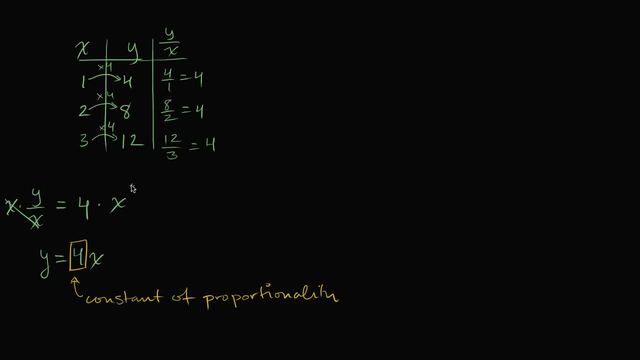 Now, sometimes it might even be described as a rate of change. You're like: well, Sal, how is this a? how would four be a rate of change? And to make that a little bit clearer, let me actually do another example. 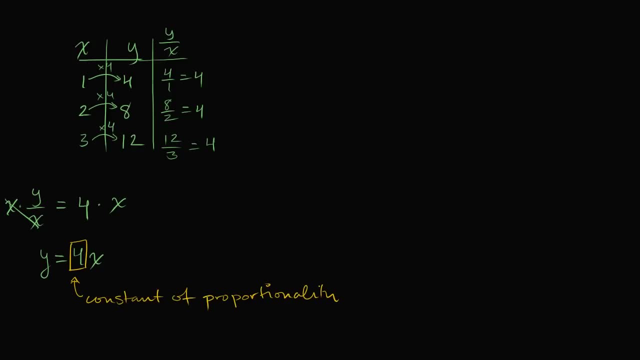 but this time I'll actually put some units there. So let's say that. let's say that I have. let's say that x. let me do this. I already used yellow. Let me use blue. So let's say x. let's say that's a measure of time. 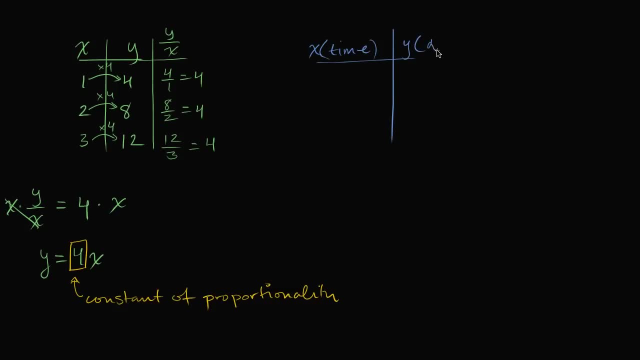 And y is a measure of distance. Or let me put it this way: x is time in terms of seconds. Let me write it this way: So x, x is going to be in seconds and then y is going to be in meters. 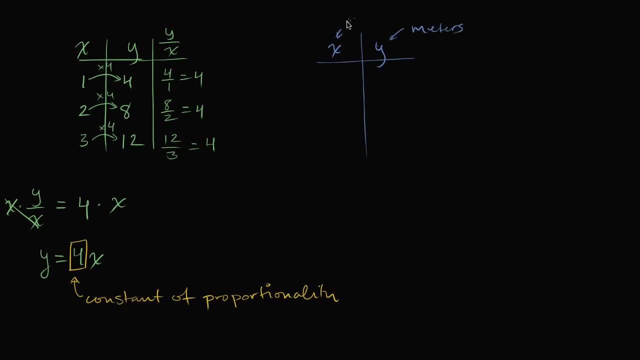 So this is meters, the units, and this right over here is seconds. So after one second we have traveled- I don't know- seven meters. After two seconds we've traveled 14 meters. After three seconds we've traveled 21 meters. 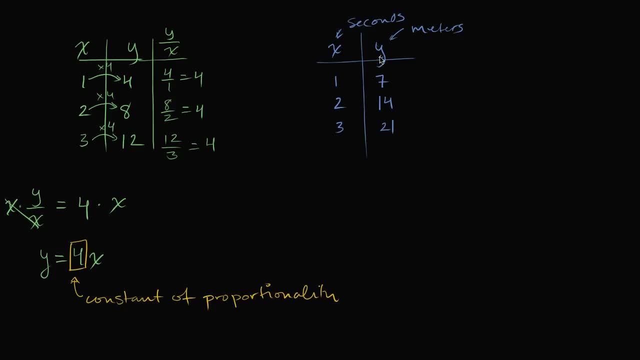 And you can verify that this is a proportional relationship. The ratio between y and x is always seven, Seven over one, 14 over two, 21 over three. But I want to write that in terms of its units. So y over x is going to be: 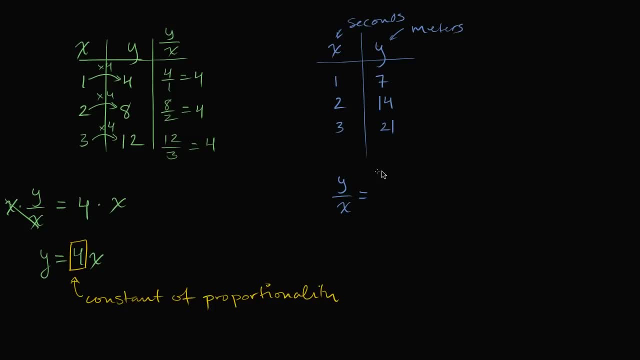 if we look at this point right over here, it's seven meters over one second, Seven meters over one second, Or it's equal to seven meters per second If you look at it right over here, if you say y over x. 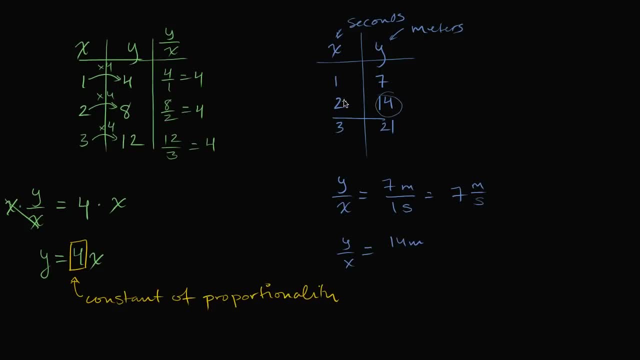 it's 14 meters. 14 meters in two seconds, in two seconds. Well, 14 over two is seven, 14 over two is seven, And then the units are meters per second. So that's why this constant, this seven, in all of these cases.